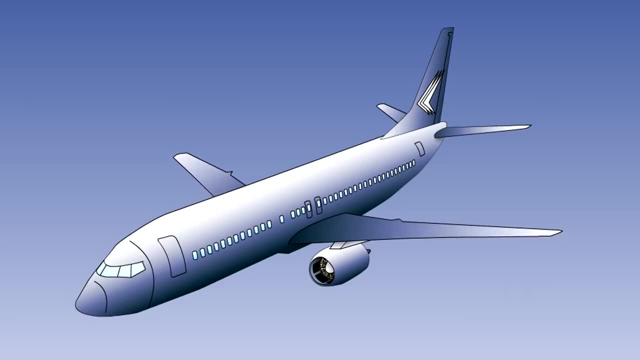 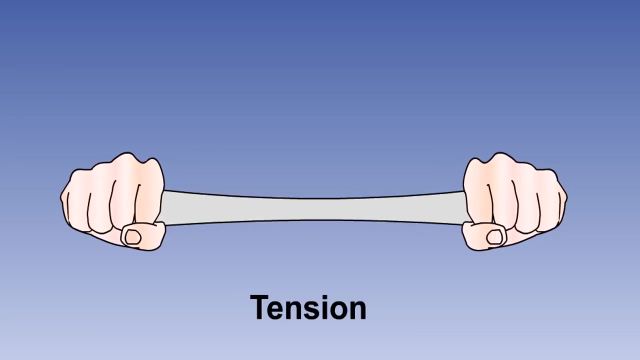 We will examine the effect of fatigue on structures and discuss the methods used to mitigate these effects. A tensile load is one which tends to stretch a structural member. The member is then said to be under tension. Components designed to resist tensile loads are known as ties. 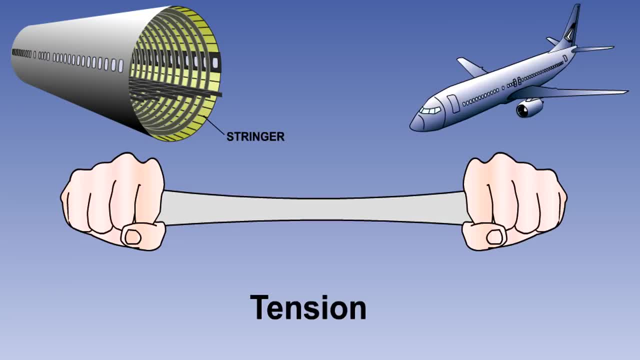 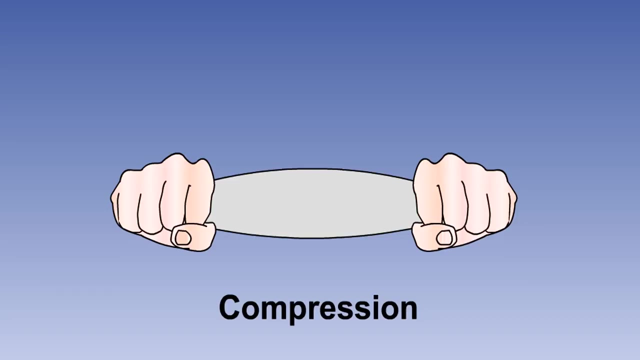 Good examples of ties are the stringers which, in modern aircraft, take the tensile loads produced in the fuselage structure by pressurization. Compressive loads are the opposite of tensile loads and tend to shorten structural members. Members subject to compressive loads are said to be under compression. 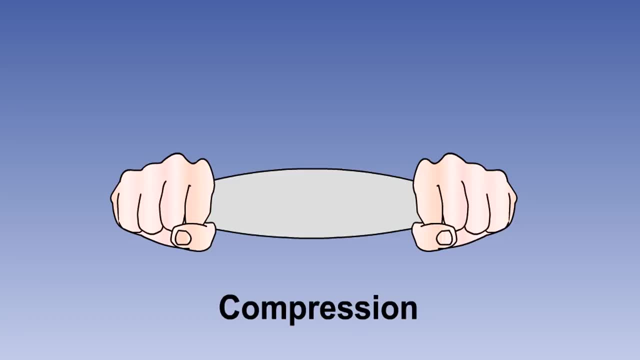 Components designed to resist compressive loads are known as struts. You will find numerous examples of struts in an aircraft landing gear, The primary one being the oleonumatic strut, which takes the compressive loads on landing. This will be fully explained in the landing gear lesson. 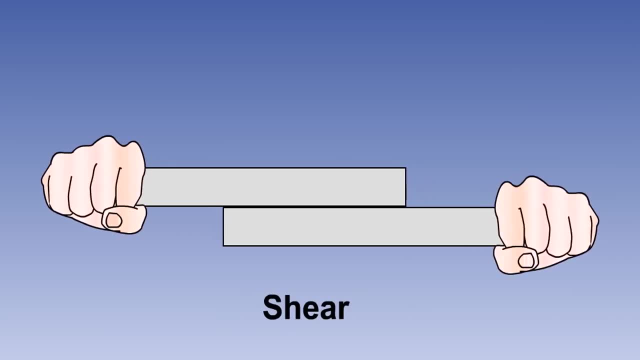 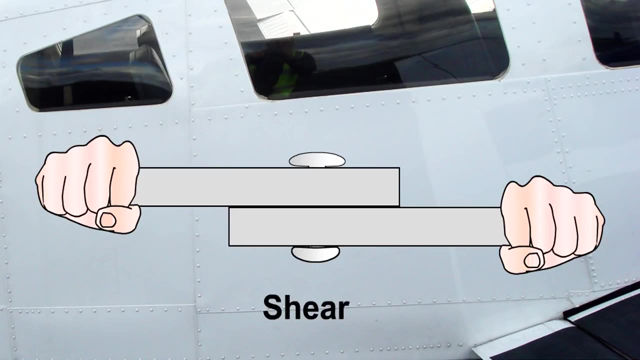 Shear is a force which tends to slide one face of the material over an adjacent face. Riveted joints are designed to resist shear forces. Rivets are being used in this picture to fasten the fuselage skin to the frame In modern aircraft. 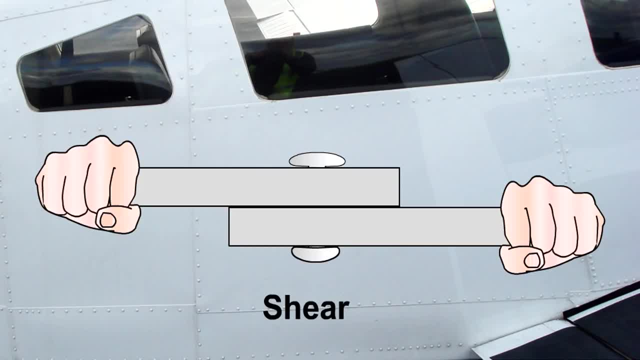 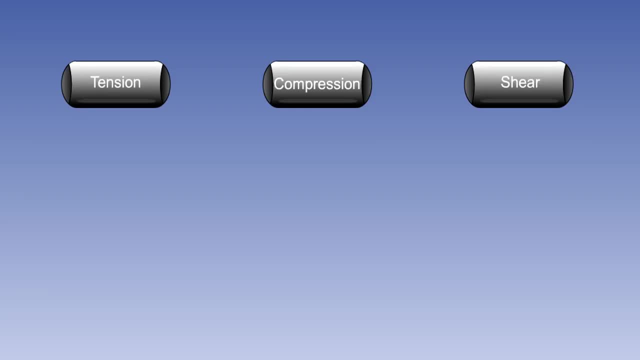 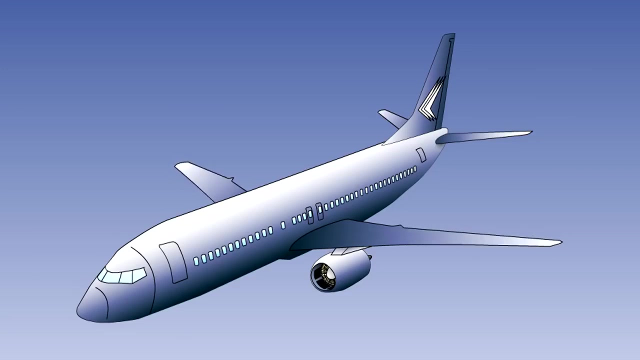 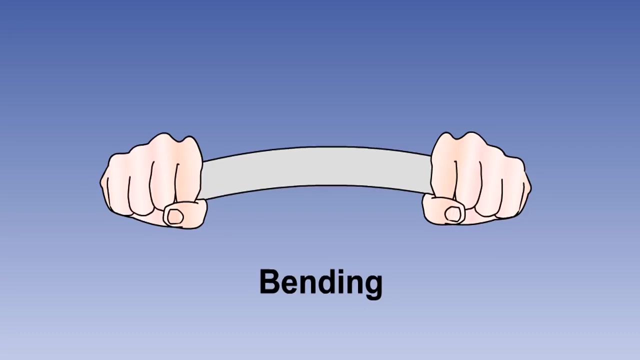 they are being replaced by adhesive bonding processes. To review tensile, compressive or shear loads, click one of the three buttons. Most loads to which aircraft components are subjected are a combination of two or all three of these basic loads. Bending of the structure involves the three basic loadings. 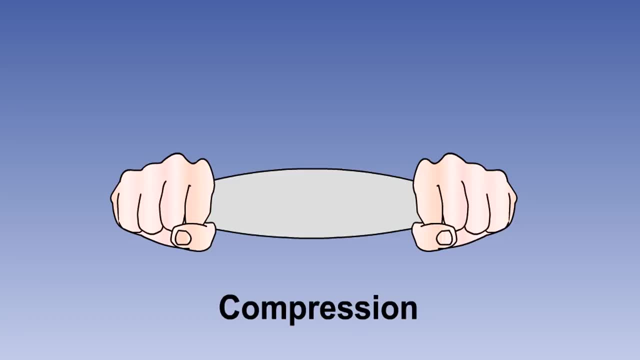 Components designed to resist compressive loads are known as struts. You will find numerous examples of struts in an aircraft landing gear, The primary one being the oleonumatic strut, which takes the compressive loads on landing. This will be fully explained in the landing gear lesson. 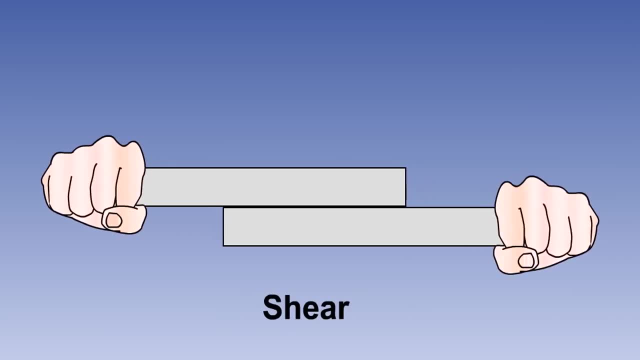 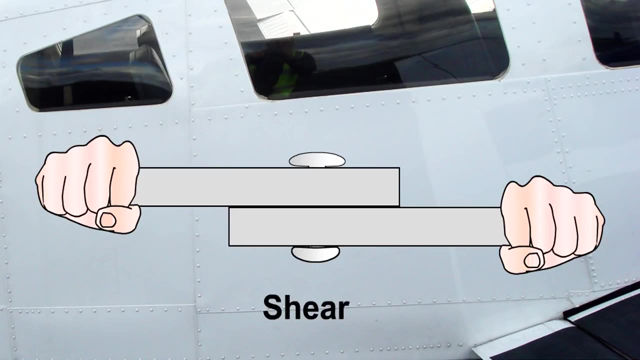 Shear is a force which tends to slide one face of the material over an adjacent face. Riveted joints are designed to resist shear forces. Rivets are being used in this picture to fasten the fuselage skin to the frame In modern aircraft. 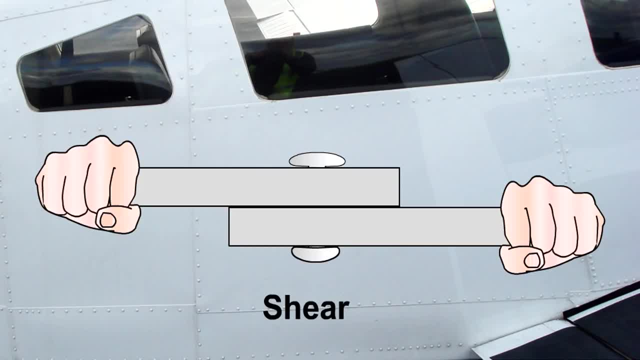 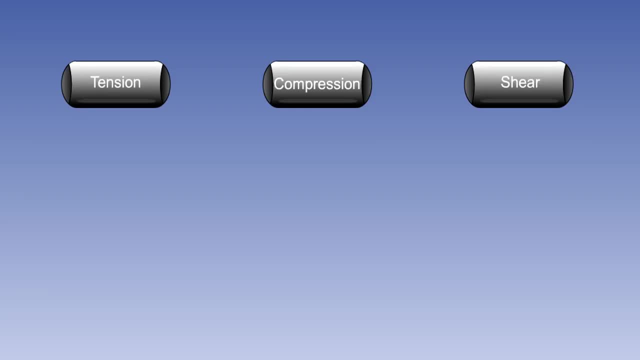 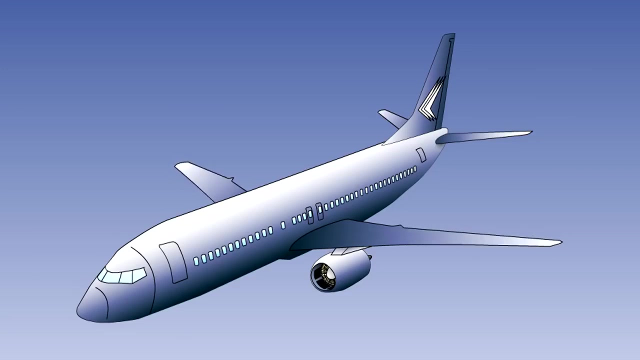 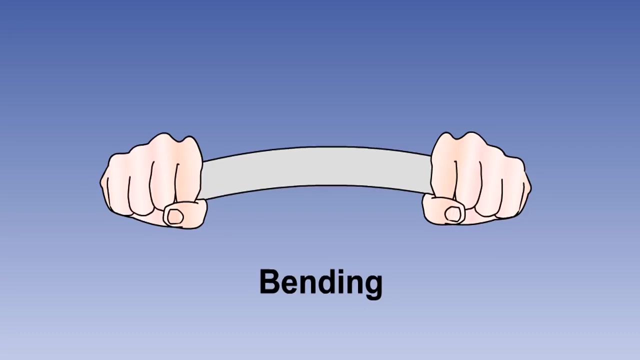 they are being replaced by adhesive bonding processes. To review tensile, compressive or shear loads, click one of the three buttons. Most loads to which aircraft components are subjected are a combination of two or all three of these basic loads. Bending of the structure involves the three basic loadings. 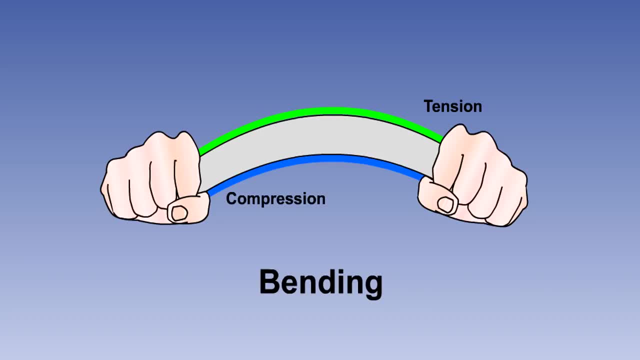 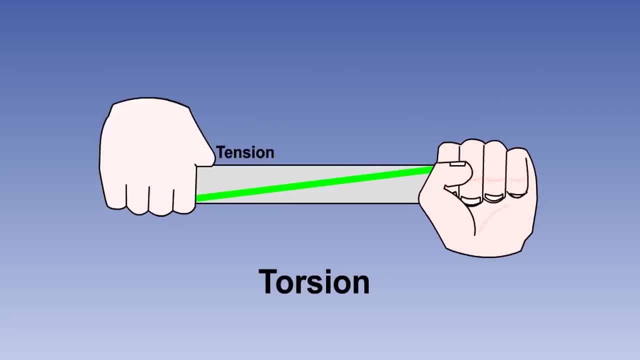 They are: tension as the outer edges stretch, compression as the inner edges squeeze together, and shear across the structure as the forces try to split it. Torsion or twisting forces produce tension at their outer edge, compression in the centre and shear forces across the structure. 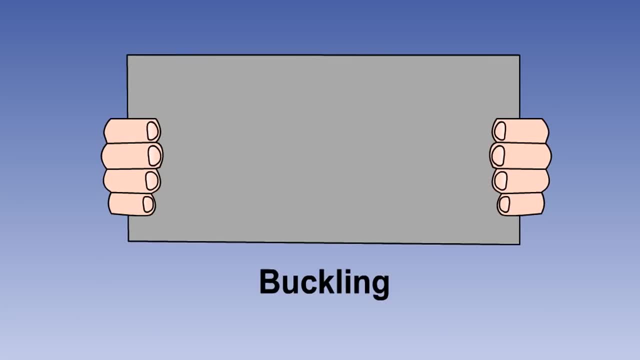 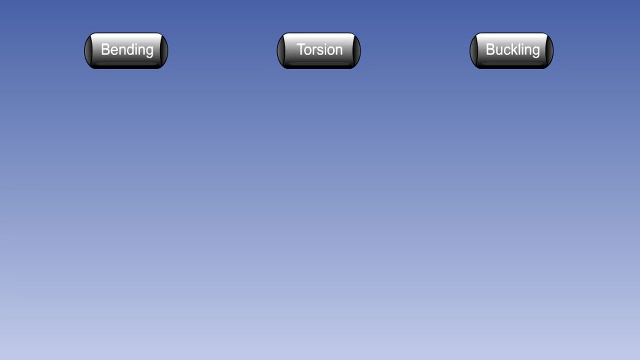 Buckling occurs to thin sheet materials when they are subjected to end loads and to ties if subjected to compressive forces. To review bending, torsion or buckling, click one of the three buttons. Stress is the internal force inside a structural member which resists an externally applied force. 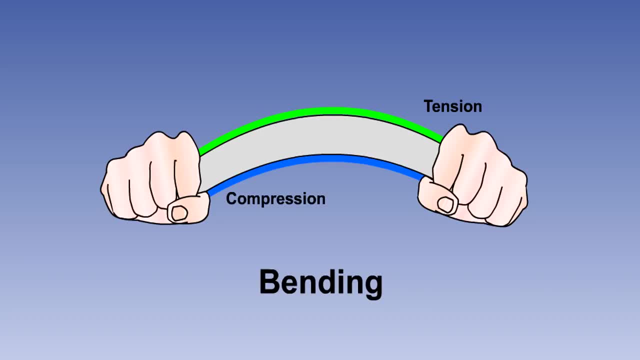 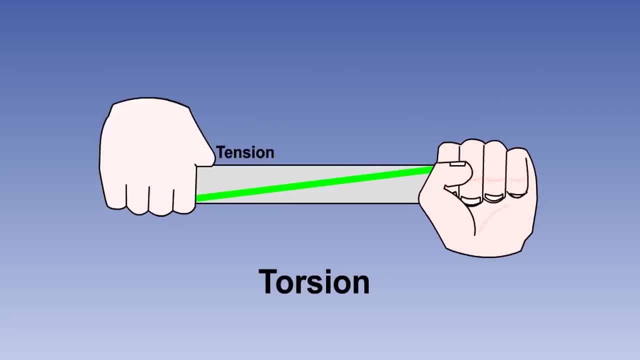 They are: tension as the outer edges stretch, compression as the inner edges squeeze together, and shear across the structure as the forces try to split it. Torsion or twisting forces produce tension at their outer edge, compression in the centre and shear forces across the structure. 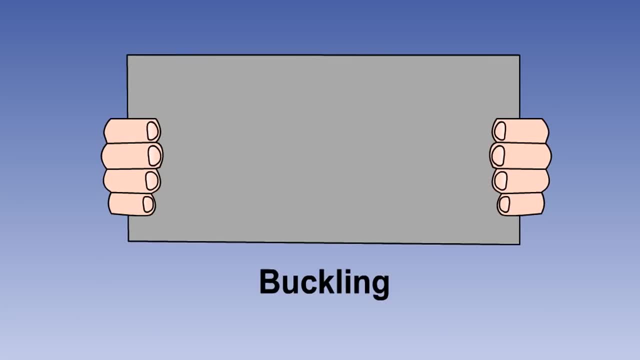 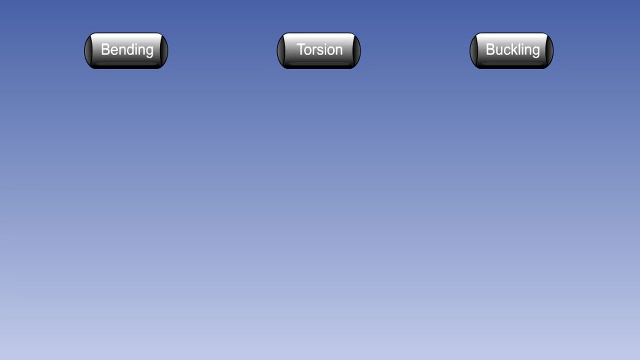 Buckling occurs to thin sheet materials when they are subjected to end loads and to ties if subjected to compressive forces. To review bending, torsion or buckling, click one of the three buttons. Stress is the internal force inside a structural member which resists an externally applied force. 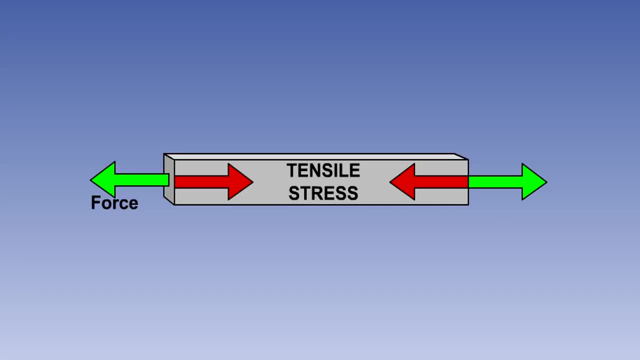 And therefore a tensile load or force will set up a tensile stress And a compressive load. compressive stress Stress is defined as the force per unit area and is measured in newtons per square millimetre Or meganewtons per square metre. 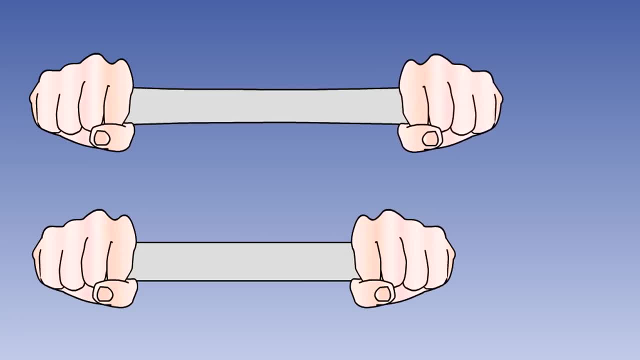 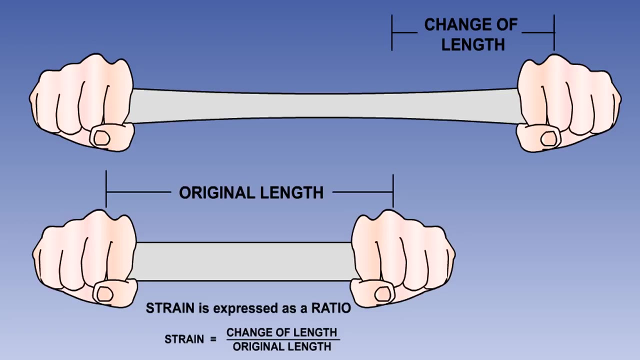 When an external force of sufficient magnitude acts on a structure, the structural dimensions change. This change is known as strain. Strain is measured as a ratio of the change in a material's length to its original length And is a measure of the deformation. 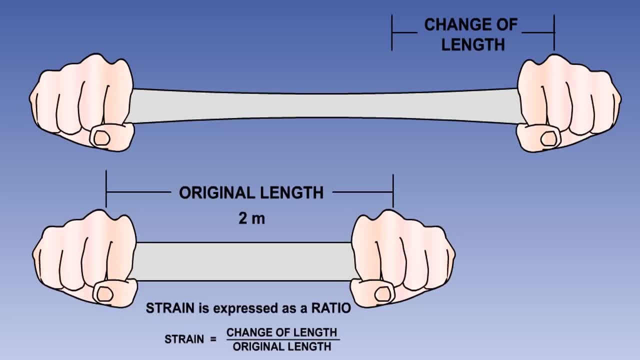 of any loaded structure. In our extreme example shown here, the original length of the material is 2 metres. When a tensile load is applied, its length increases to 2.5 metres. This gives it an increase in length of 0.5 metres. 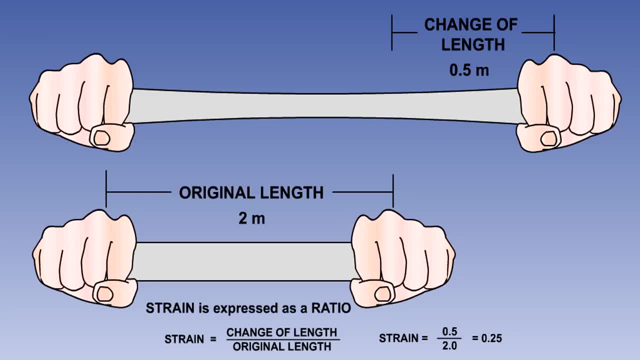 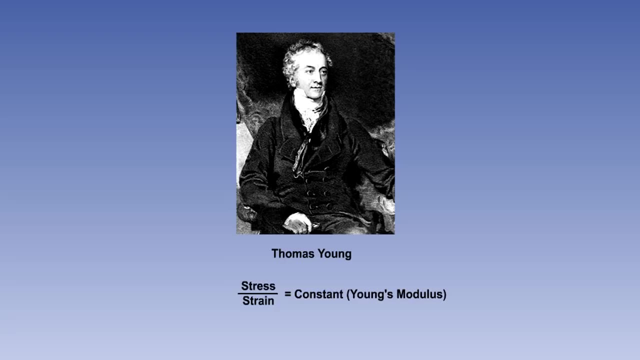 Therefore, the strain being felt by this material is 0.5 divided by 2, which is 0.25.. The 18th century English physicist, Thomas Young, discovered that the relationship between stress and strain for an elastic material within the elastic limit of the material. 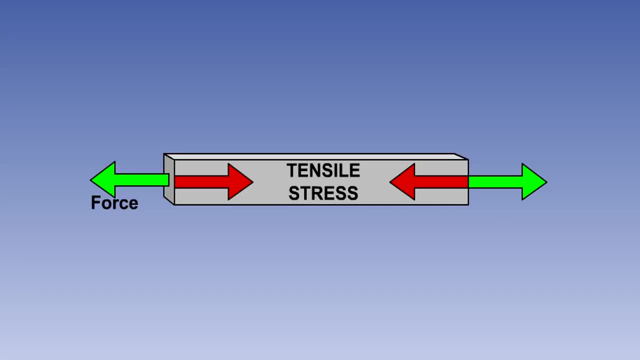 And therefore a tensile load or force will set up a tensile stress And a compressive load. compressive stress Stress is defined as the force per unit area and is measured in newtons per square millimetre Or meganewtons per square metre. 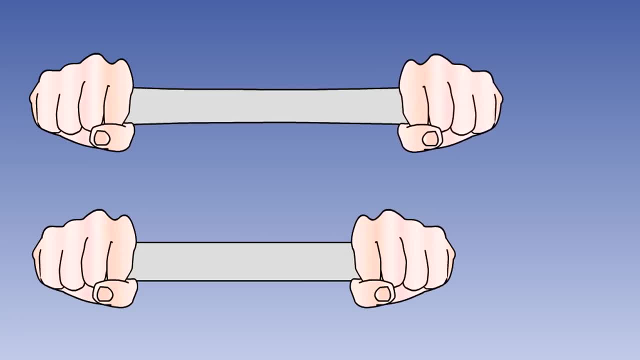 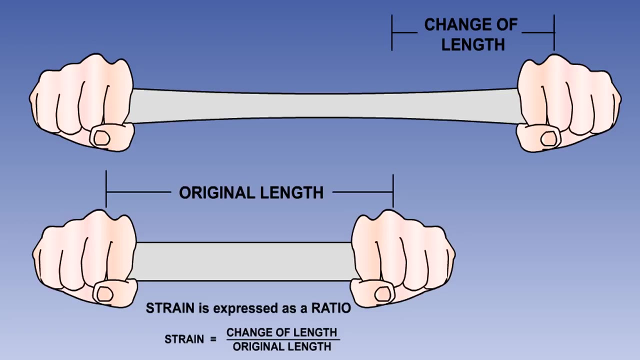 When an external force of sufficient magnitude acts on a structure, the structural dimensions change. This change is known as strain. Strain is measured as a ratio of the change in a material's length to its original length And is a measure of the deformation. 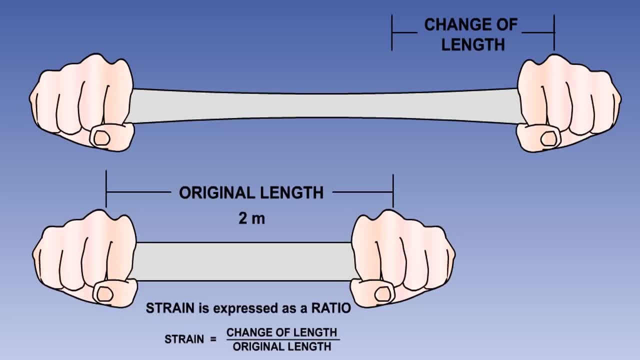 of any loaded structure. In our extreme example shown here, the original length of the material is 2 metres. When a tensile load is applied, its length increases to 2.5 metres. This gives it an increase in length of 0.5 metres. 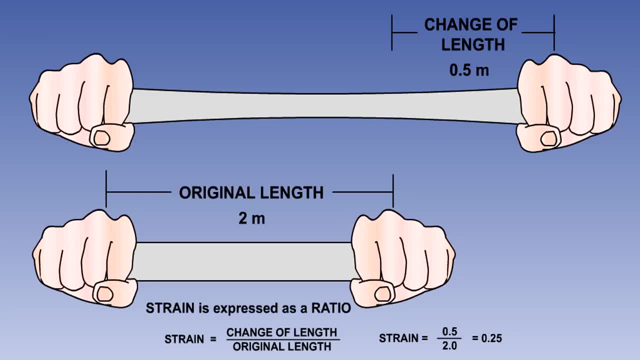 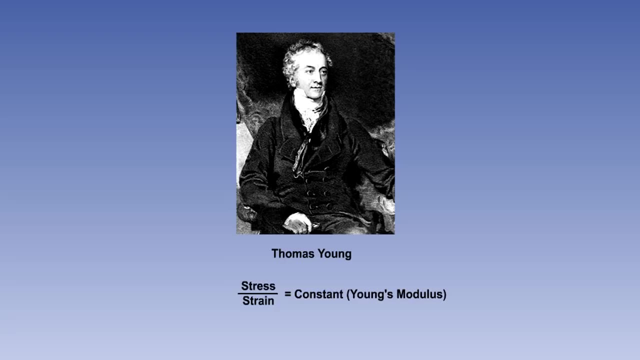 Therefore, the strain being felt by this material is 0.5 divided by 2, which is 0.25.. The 18th century English physicist, Thomas Young, discovered that the relationship between stress and strain for an elastic material within the elastic limit of the material. 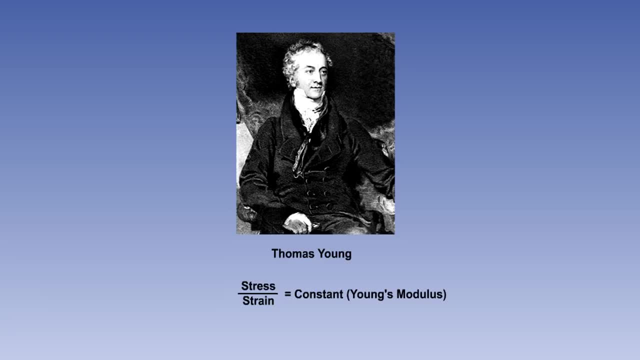 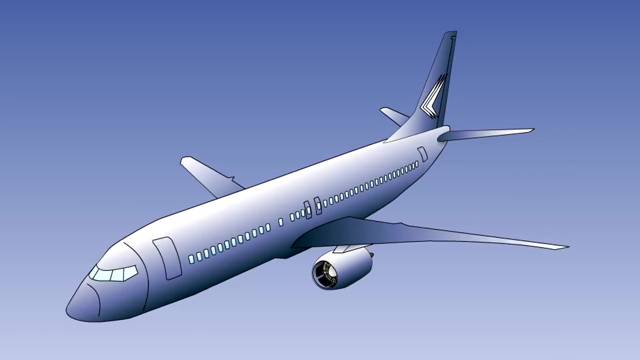 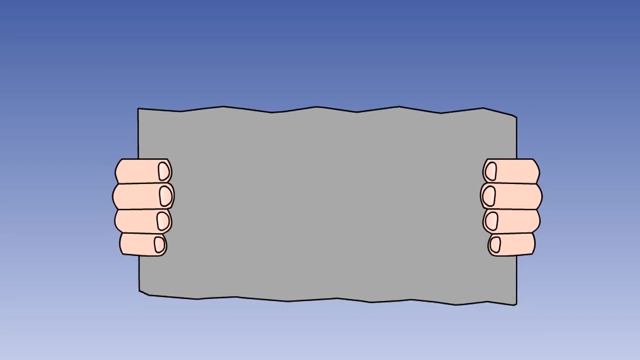 is generally a constant. This constant is therefore known as Young's modulus of elasticity. Aircraft components are subjected to some or all of these stresses, and they will tend to elongate, compress, bend, shear and twist the component. However, provided the deformation is within 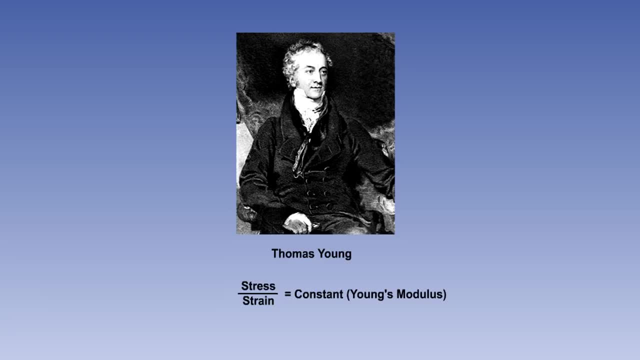 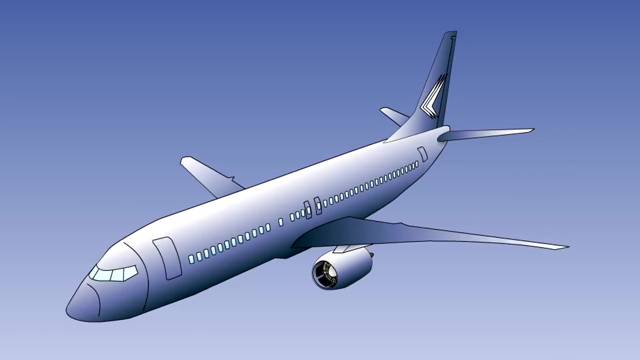 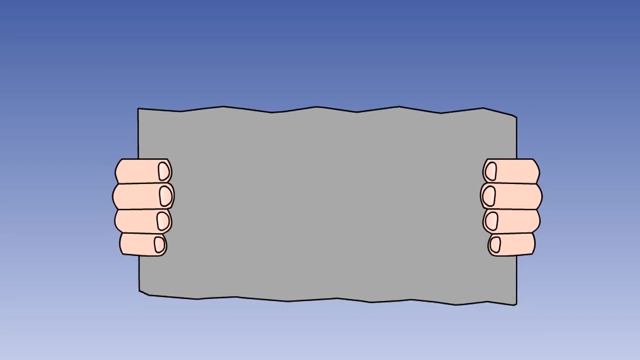 is generally a constant. This constant is therefore known as Young's modulus of elasticity. Aircraft components are subjected to some or all of these stresses, and they will tend to elongate, compress, bend, shear and twist the component. However, provided the deformation is within 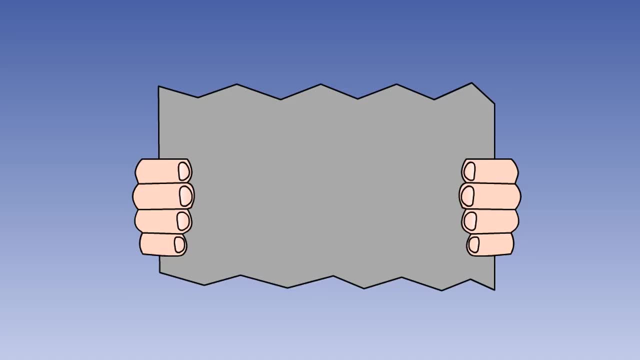 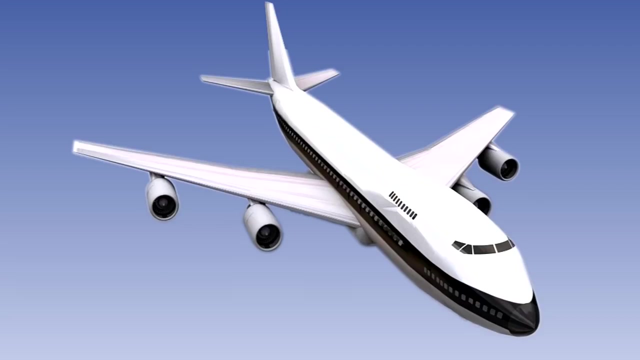 the elastic limit of the material. the component will return to its original dimension once the stress has been removed. If any load takes the structure beyond its elastic limit, then the deformation will be permanent. The maximum load that a designer would expect: an airframe or component. 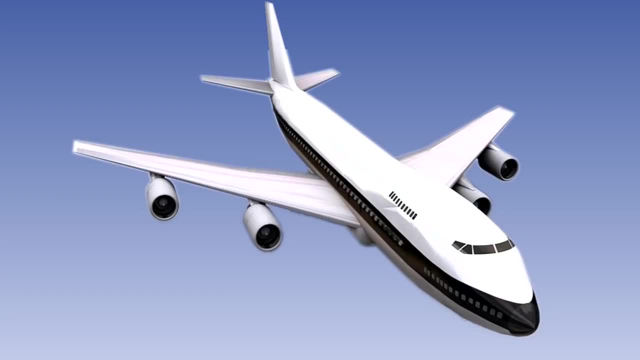 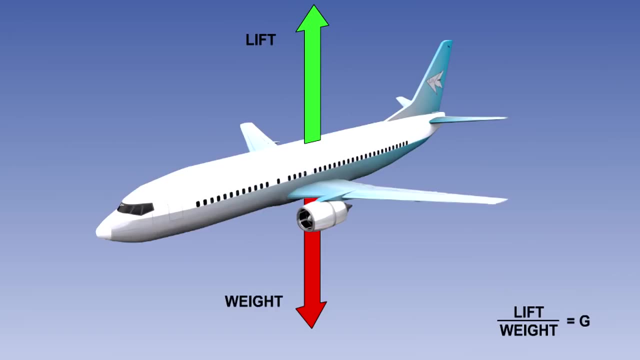 to experience in service is termed the design limit load. This load is defined as a load factor. The load factor is the ratio of the lift of an aircraft to the weight of the aircraft. The load factor is expressed in multiples of g In straight and level flight. 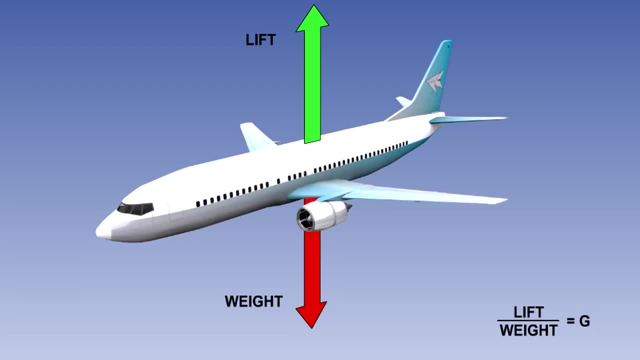 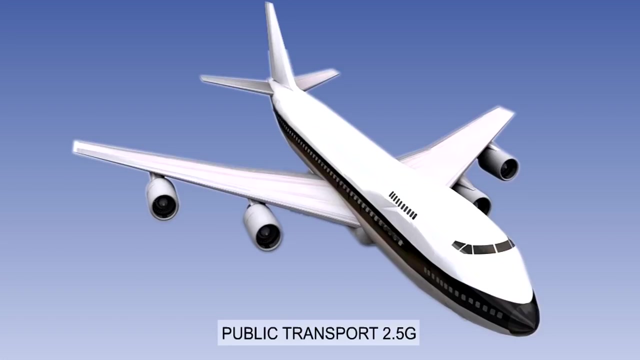 lift is equal to weight. so the ratio of lift to weight is 1, and the load factor is 1g. The load factor is expressed in multiple of g. The design limit load is 2.5G for public transport aeroplanes. 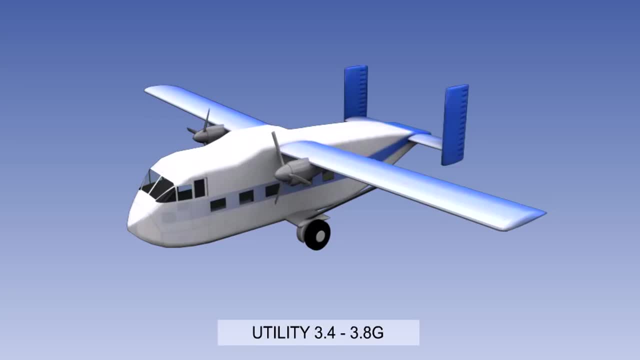 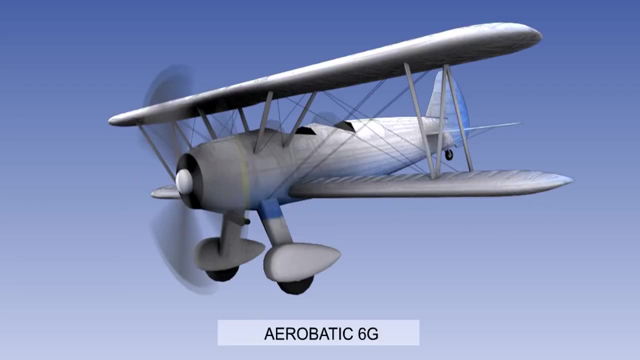 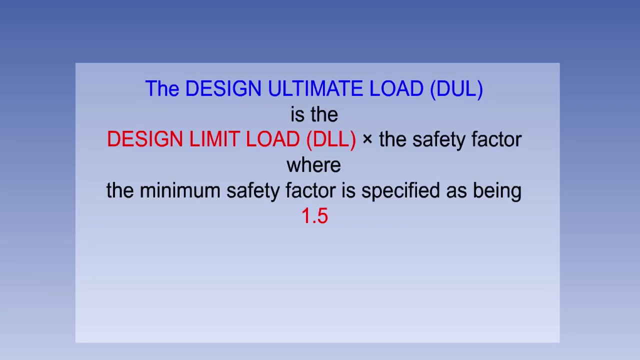 The design limit load is 3.4 to 3.8G for utility aircraft and 6G for aerobatic aircraft. The design ultimate load is the design limit load multiplied by a safety factor. The minimum safety factor specified in design requirements is 1.5.. 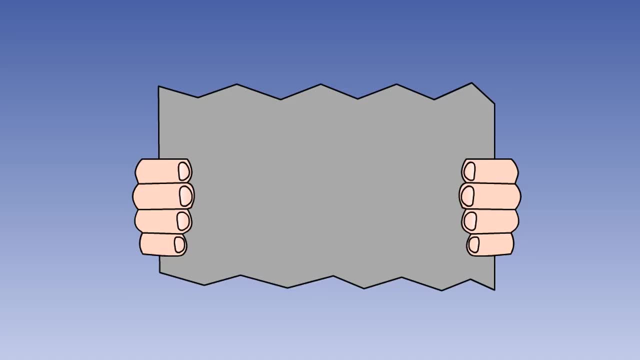 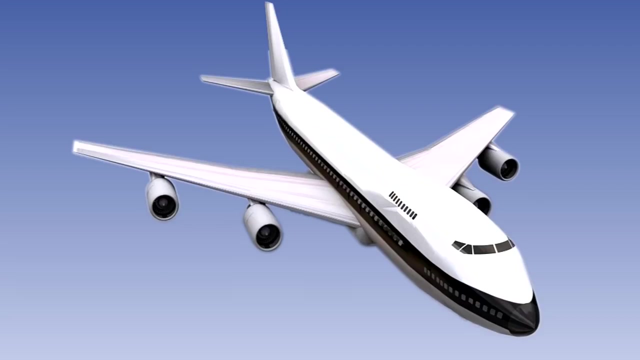 the elastic limit of the material. the component will return to its original dimension once the stress has been removed. If any load takes the structure beyond its elastic limit, then the deformation will be permanent. The maximum load that a designer would expect: an airframe or component. 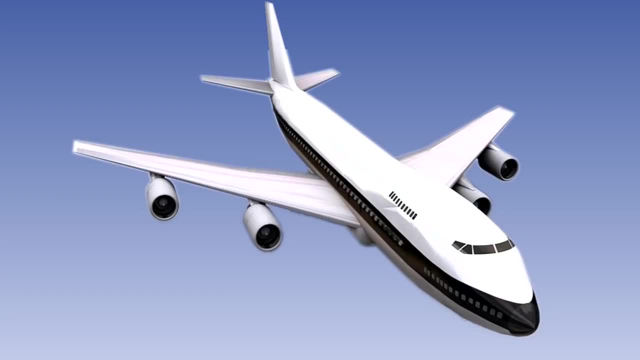 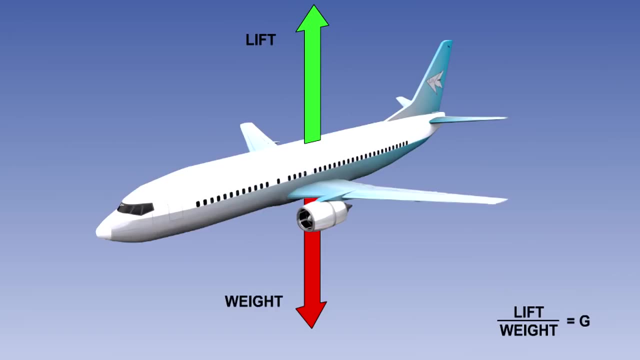 to experience in service is termed the design limit load. This load is defined as a load factor. Load factor is the ratio of the lift of an aircraft to the weight of the aircraft. The load factor is expressed in multiples of g In straight and level flight. 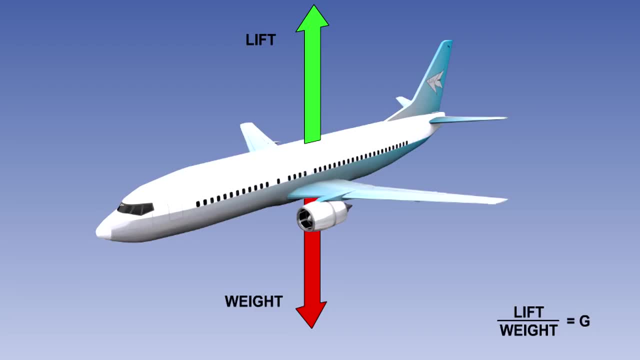 lift is equal to weight, so the ratio of lift to weight is 1, and the load factor is 1 g. In linear and longitudinal flight, the load factor is 0.5 g. Thus the load factor is 1 g. 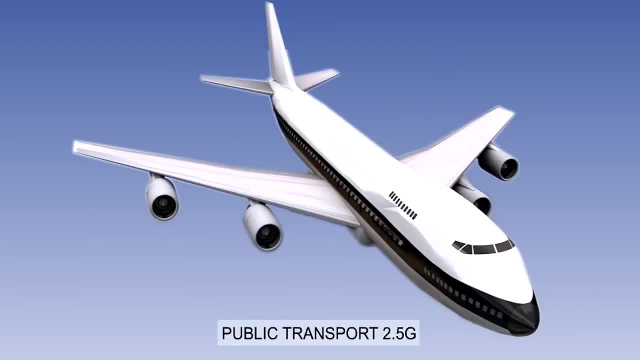 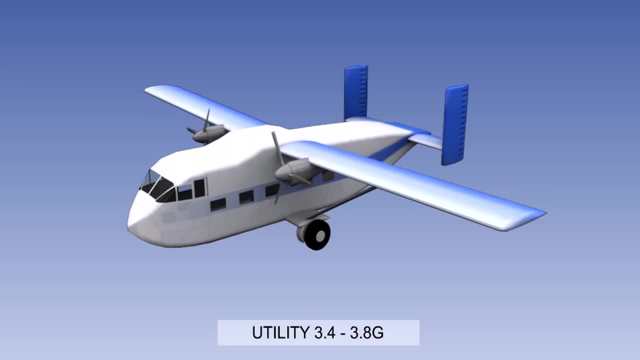 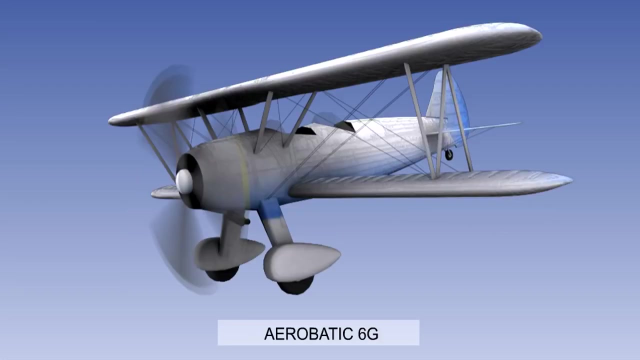 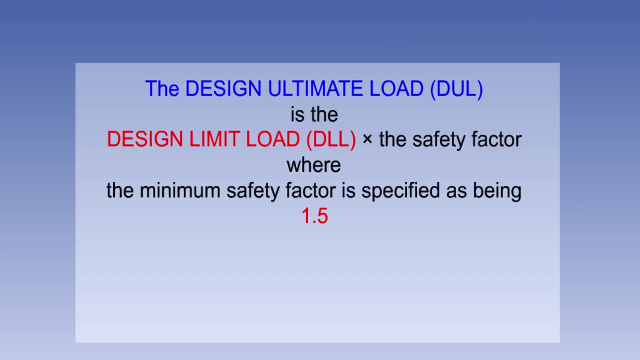 The design limit load is 2.5G for public transport aeroplanes. The design limit load is 3.4 to 3.8G for utility aircraft and 6G for aerobatic aircraft. The design ultimate load is the design limit load multiplied by a safety factor. 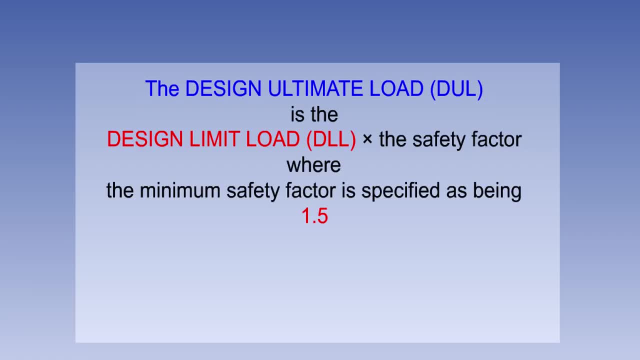 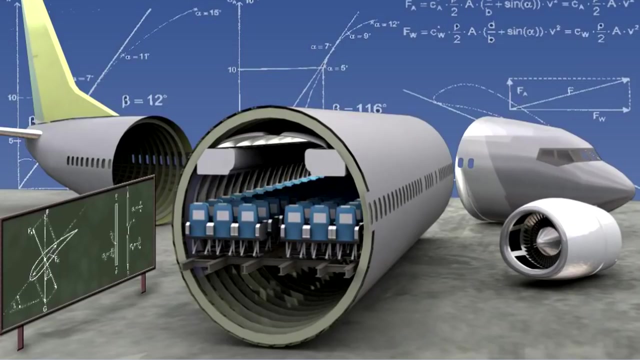 The minimum safety factor specified in design requirements is 1.5.. The structure must withstand its design ultimate load without collapse. The safety factor is the ratio of the design ultimate load to the design limit load. The aircraft manufacturer will attempt to design an aircraft. 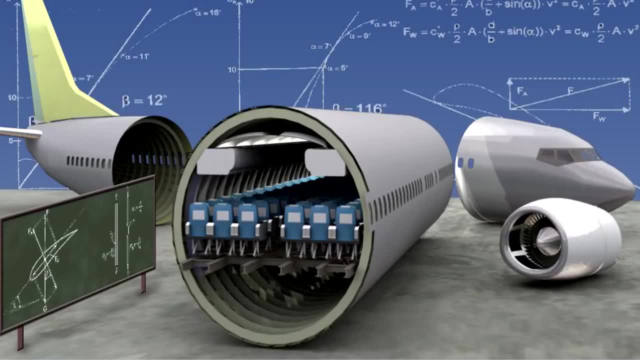 to take into account all the loads that it may experience in flight. There are various guidelines, formula and experience to help them in the design of good, fail-safe and damage-tolerant structures. The designer will take into account the anticipated role of the aircraft. so, for instance, aircraft 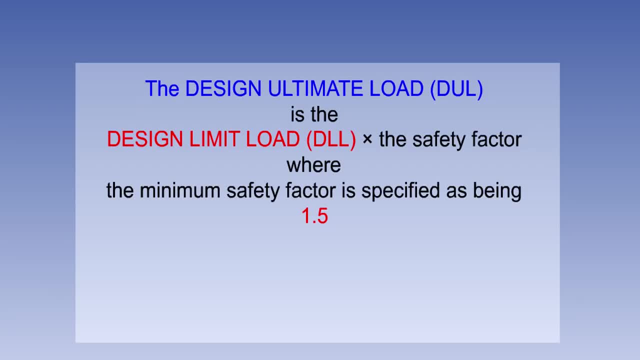 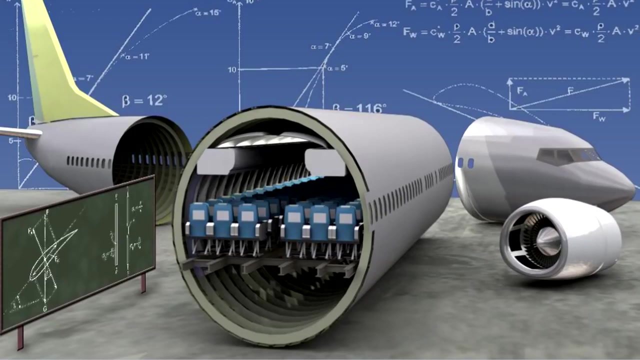 The structure must withstand its design ultimate load without collapse. The safety factor is the ratio of the design ultimate load to the design limit load. The aircraft manufacturer will attempt to design an aircraft to take into account all the loads that it may experience in flight. 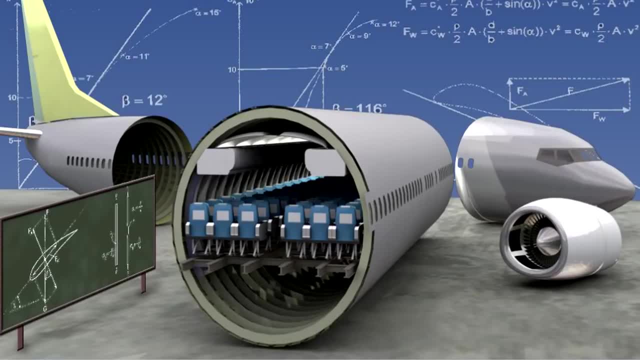 There are various guidelines, formula and experience to help them in the design of good, fail-safe and damage-tolerant structures. The designer will take into account the anticipated role of the aircraft. so, for instance, aircraft designed for long-haul operations should not be used for short-haul, as the extra take-offs 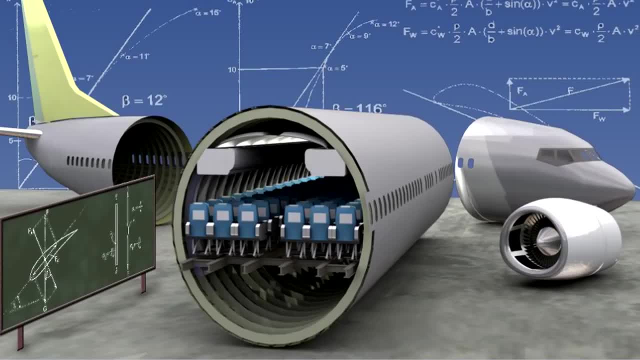 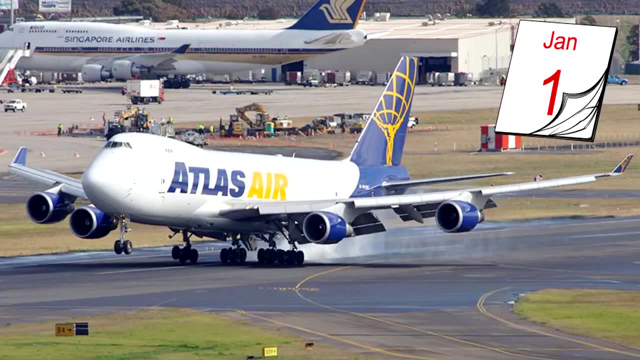 and landings. The aircraft will not have been accounted for in the airframe's anticipated fatigue life calculations. The safe life of an aircraft structure is defined as the minimum life during which it is known that no catastrophic failure will occur. All critical components have a safe life, which may be measured in flying hours, landings. 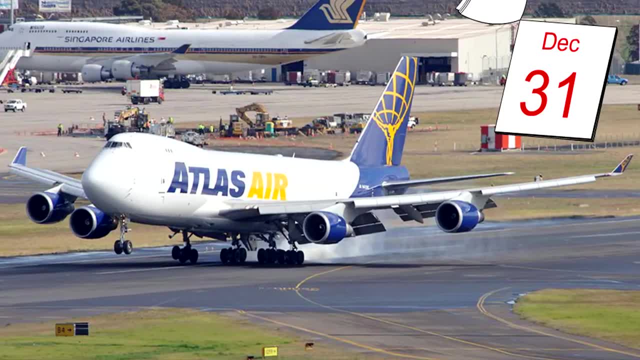 pressurization cycles or even on a calendar basis. After the permitted safe life count has been reached, the relevant item is replaced or overhauled During the operational life of the aircraft. to minimize the effects of mental fatigue, aircraft designers apply the principles of fail-safe or damage-tolerant construction. 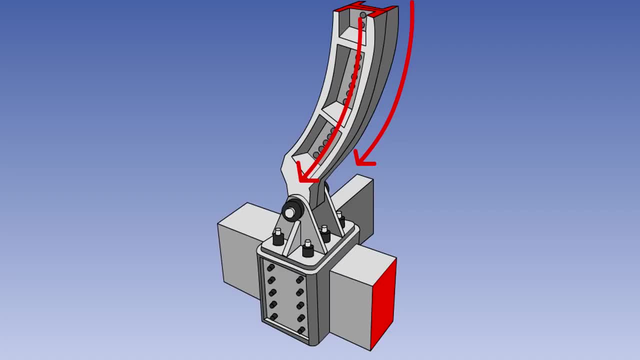 A fail-safe structure is based on the principle of component redundancy. It has a maximum capacity of a single aircraft. It has multiple load paths in parallel, which means that the loads are shared by adjacent members. Therefore, if one part fails, the load will be carried by the adjacent member for a limited. 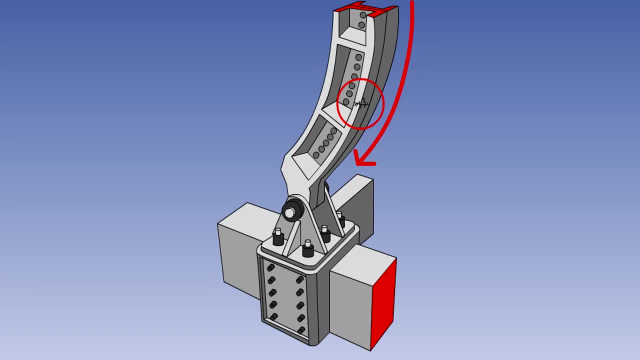 period. This must be until at least the next periodic inspection. The disadvantage of duelling the load paths is that it is very expensive in terms of weight, as each of them has a maximum capacity. The return load is known to be over a key part of the union. In the future, the user may need to use a new load path to replace it. It has to be a double-layer load path that makes it possible to use the load path. It must be made in a manner the user is familiar with the load path process and the use of. 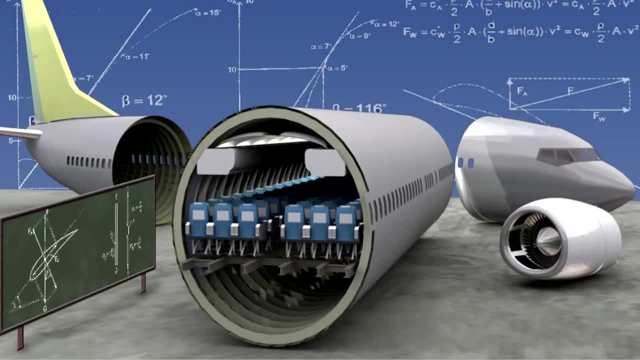 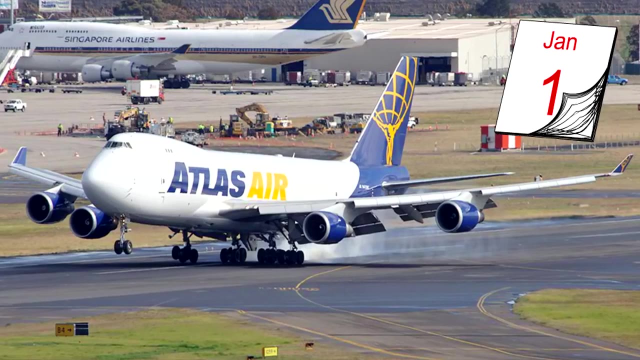 designed for long-haul operations should not be used for short-haul, as the extra take-offs and landings The aircraft will not have been accounted for in the airframe's anticipated fatigue life calculations. The safe life of an aircraft structure is defined as the minimum life during which it 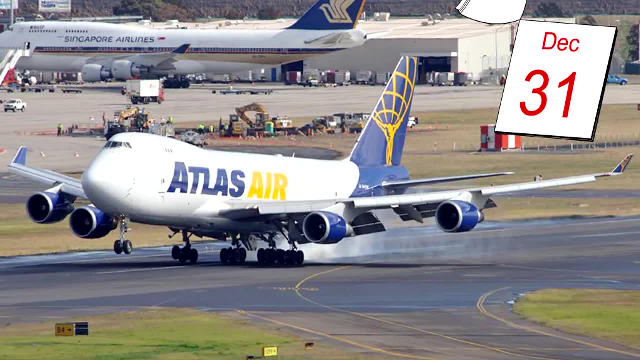 is known that no catastrophic failure will occur. All critical components have a safe life, which may be measured in flying hours, landings, pressurization cycles or even on a calendar basis. After the permitted safe life count has been reached, the relevant item is replaced or. 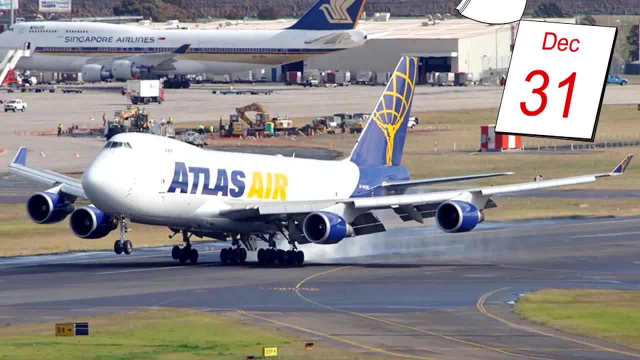 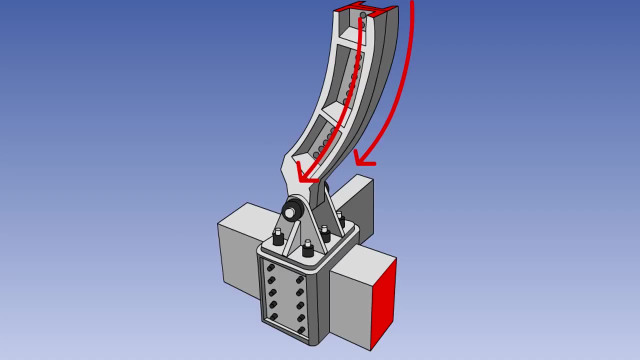 overhauled During the operational life of the aircraft. to minimize the effects of mental fatigue, aircraft designers apply the principles of fail-safe or damage-tolerant construction. A fail-safe structure is based on the principle of component redundancy. It has a maximum capacity of a single aircraft. 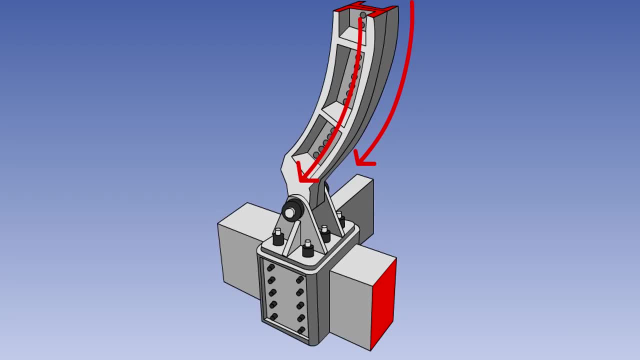 It has multiple load paths in parallel, which means that the loads are shared by adjacent members. Therefore, if one part fails, the load will be carried by the adjacent member for a limited period. This must be until at least the next periodic inspection. 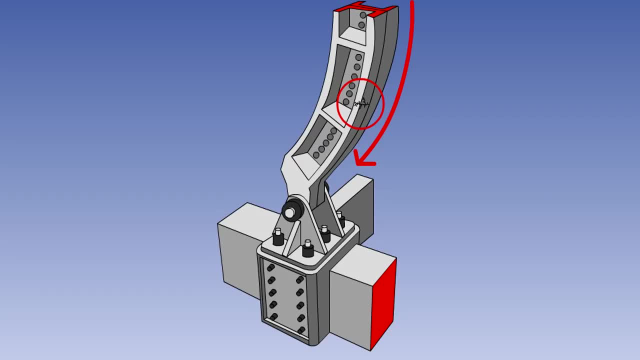 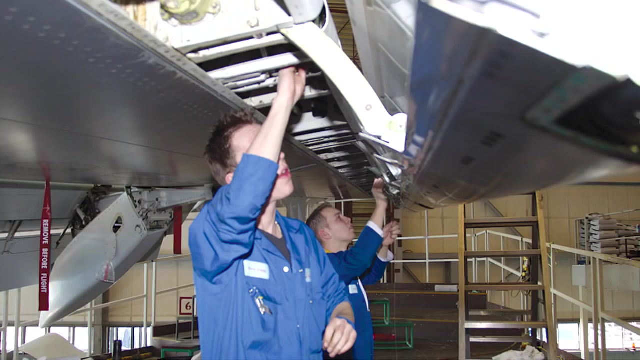 The disadvantage of duelling the load paths is that it is very expensive in terms of weight, as each of them has a maximum capacity. The weight of the load path between the wings can be a Heinrich von No 없 Equipment Pros Cons tr profundization. 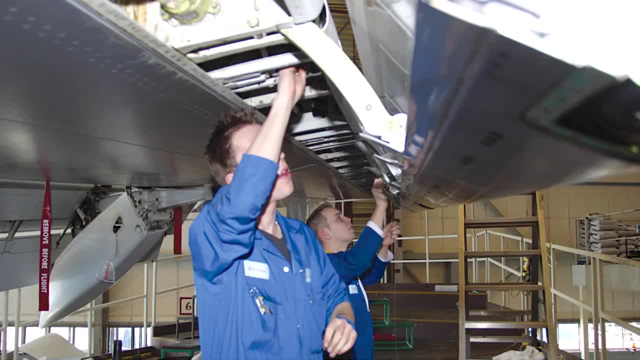 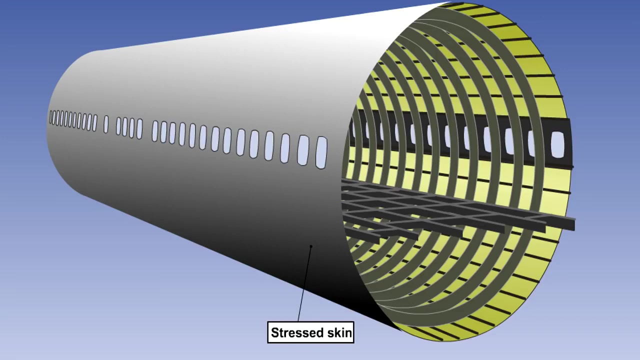 Pairs to ensure that failures are detected before they progress too far. To gain access to vulnerable areas, a certain amount of dismantling is usually required, although non-destructive testing may be used in less critical areas. Modern concepts of aircraft design employ the stressed skin style of construction. 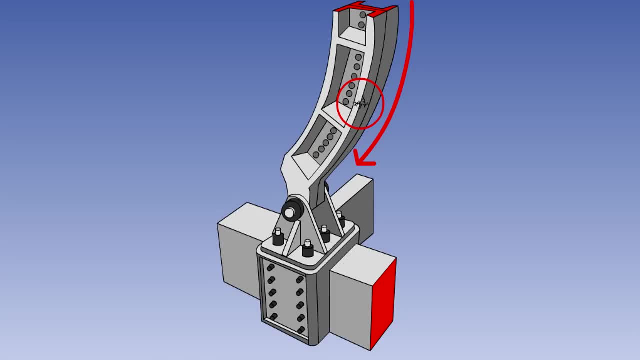 the load path loss factor. The load path costs the user a considerable amount of time. A load path may be a two-day load at any time and it requires extra time to save time. The load path is the same after the construction of the load path. 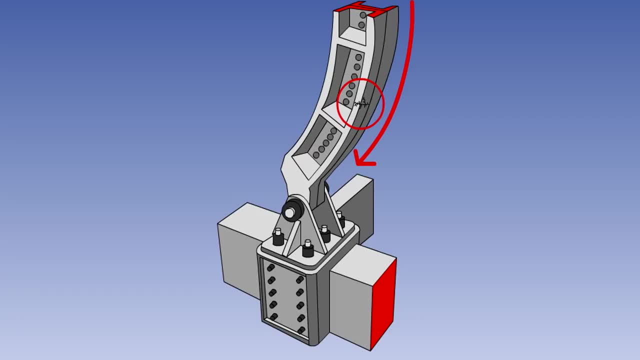 If you make the restricted load path, the load path will be damaged after the construction of the load path. It is not necessary to use a load path in a two-day or three-day load path. The load path must be a minimum of two minutes, depending on your type of load path. 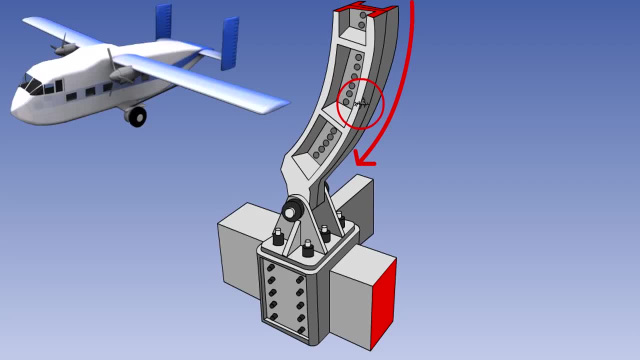 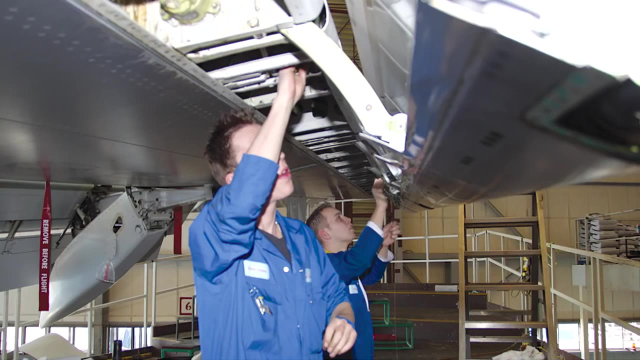 The bracing struts between the wings and the fuselage of the short sky van, for instance, are each made up of three members. This design philosophy must be accompanied by a maintenance program to ensure that failures are detected before they progress too far. 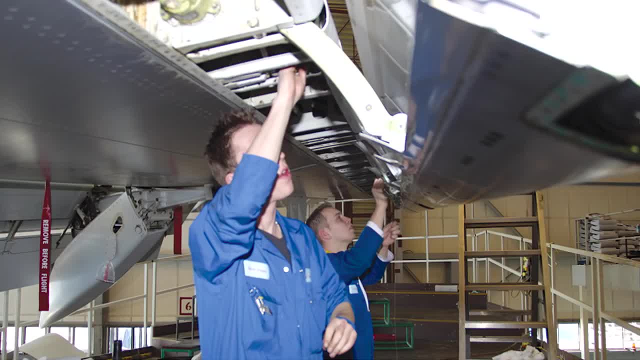 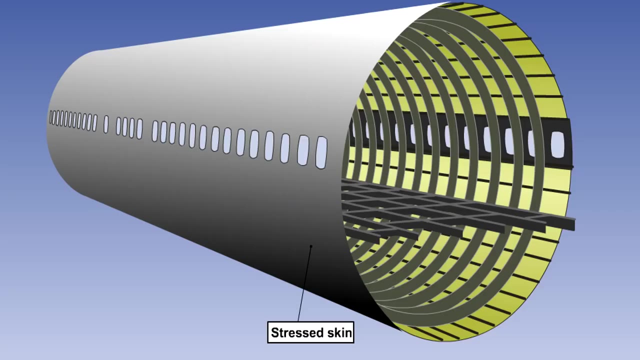 To gain access to vulnerable areas, a certain amount of dismantling is usually required, although non-destructive testing may be used in less critical areas. Modern concepts of aircraft design employ the stressed skin style of construction, where each piece of the airframe, including the stressed skin, plays its part in spreading loads throughout. 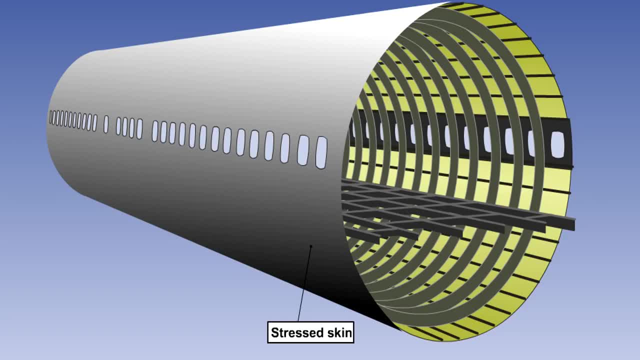 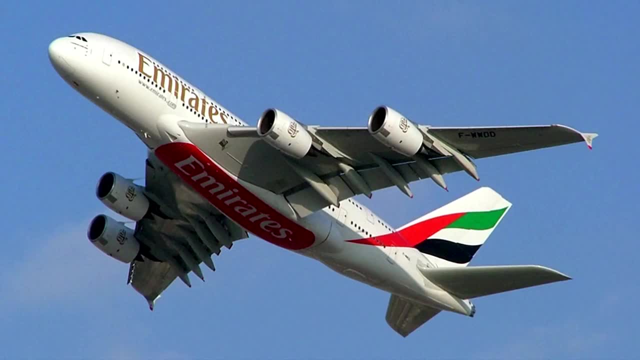 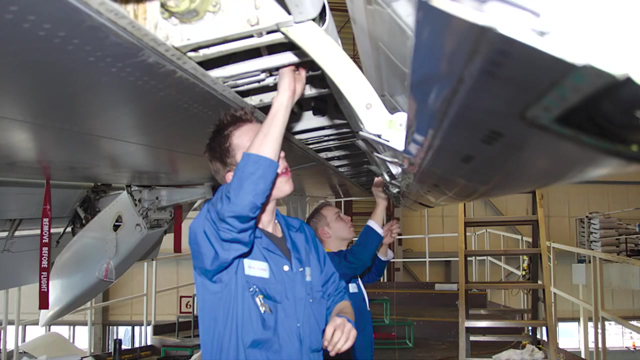 The entire airframe is tolerant to a certain amount of damage. These damage-tolerant structures eliminate the extra structural members needed in a fail-safe design by spreading the loading of a particular structure over a larger area. Damage-tolerant structures are designed to withstand a certain amount of damage. 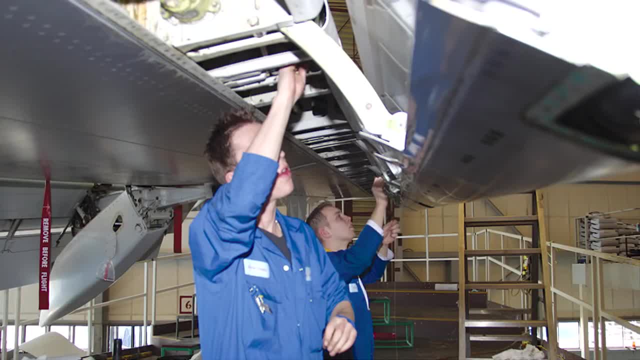 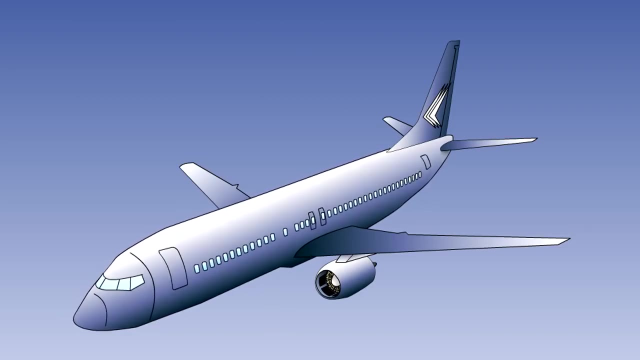 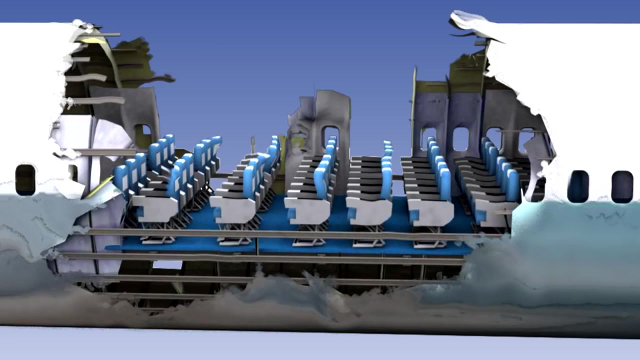 which again should be detected during the normal inspection cycle before a failure occurs. A structure which is subject to continual reversals of loading, such as the landing gear or the fuselage of a pressurized aircraft, will fail at a load of less than would be the case for a steadily applied load. 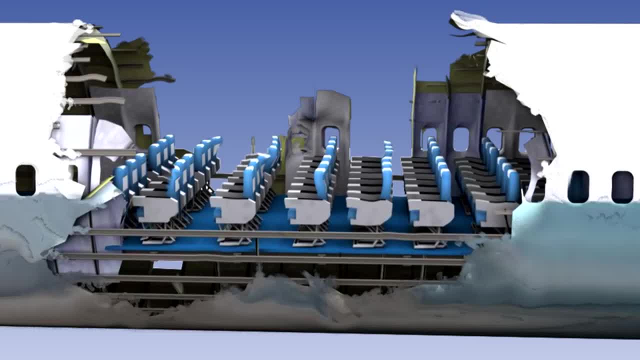 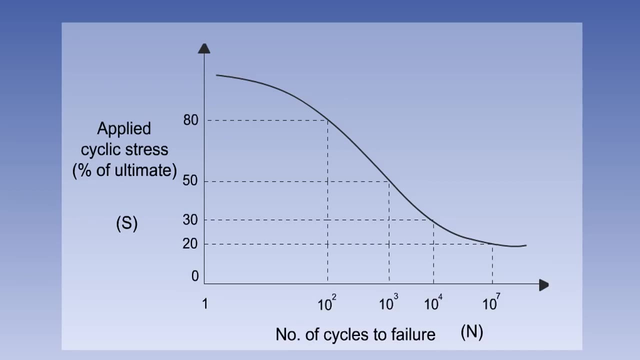 This is known as fatigue. The failure load level will decrease and will depend on the number of reversals experienced In high-cycle fatigue situations. a material performance can be graphically characterized by an S-N curve, also known as a Wöhler curve. 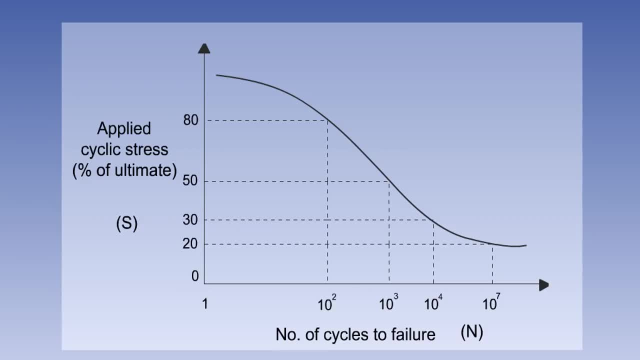 This is a graph of the magnitude of the cycle stress S against a logarithmic scale of cycles to failure N. This is a graph of the magnitude of the cycle stress S against a logarithmic scale of cycles to failure N. 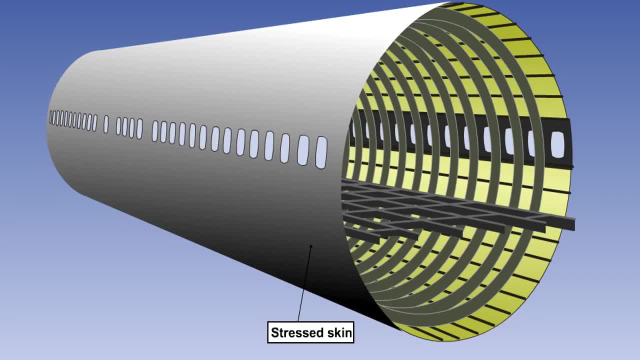 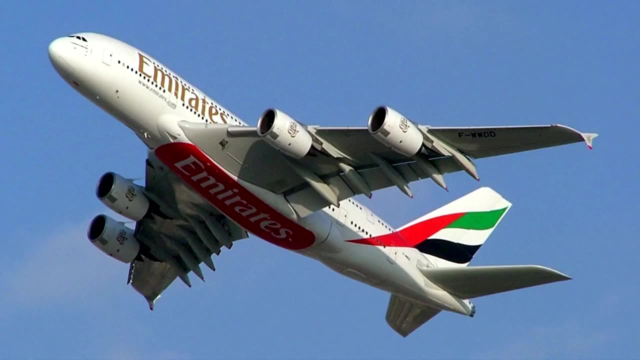 where each piece of the airframe, including the stressed skin, plays its part in spreading loads throughout the entire airframe and is tolerant to a certain amount of damage. These damage-tolerant structures eliminate the extra structural members needed in a fail-safe design. 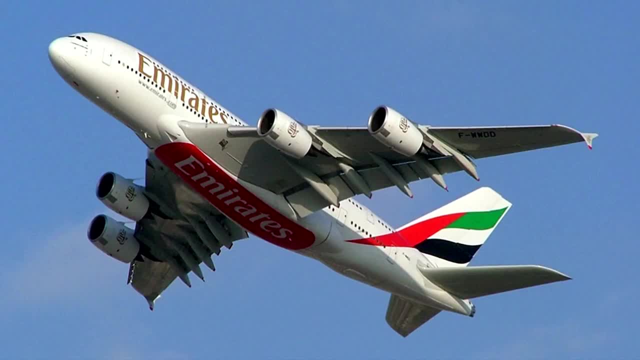 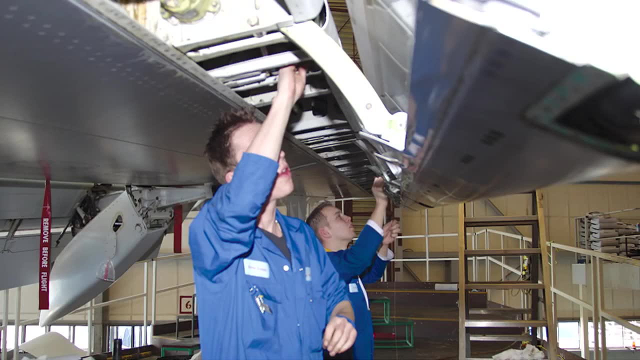 by spreading the loading of a particular structure over a larger area. Damage-tolerant structures are designed to be able to be used in a lot of different ways. They are designed to withstand a certain amount of damage, which again should be detected during the normal inspection cycle before a failure occurs. 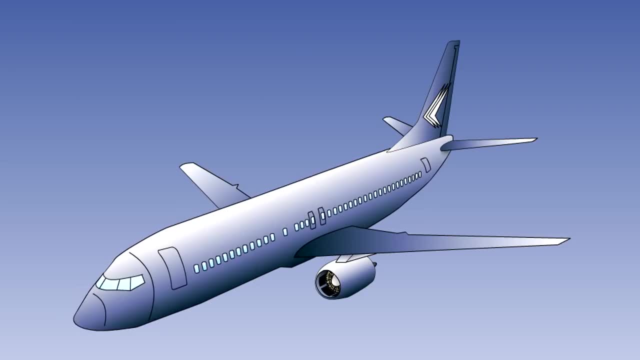 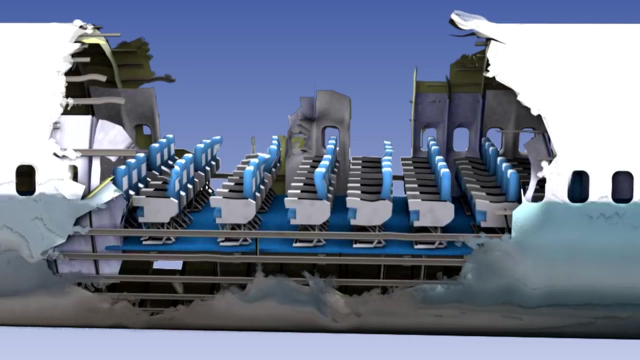 A structure which is subject to continual reversals of loading, such as the landing gear or the fuselage of a pressurised aircraft, will fail at a load of less than would be the case for a steadily applied aircraft. This is known as fatigue. 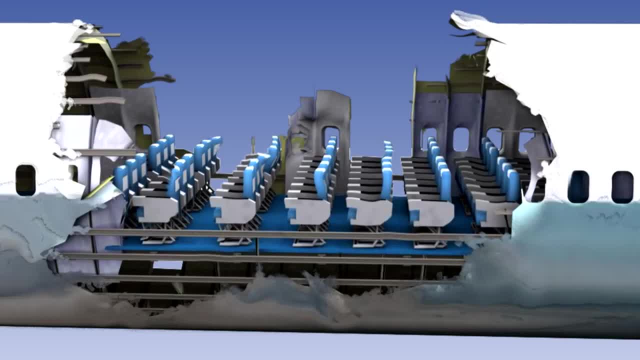 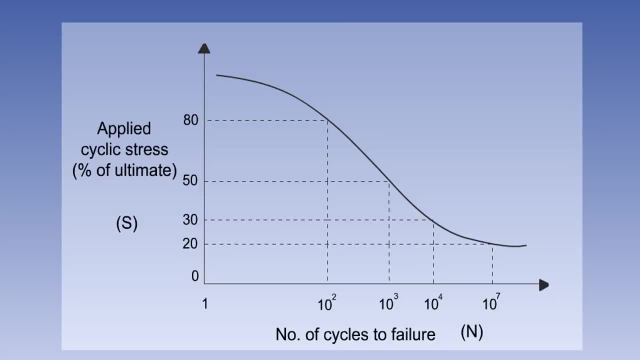 The failure load level will depend on the number of reversals experienced In high-cycle fatigue situations. a material performance can be graphically characterised by an SN curve, also known as a Vohler curve. This is a graph of the magnitude of the failure load level. 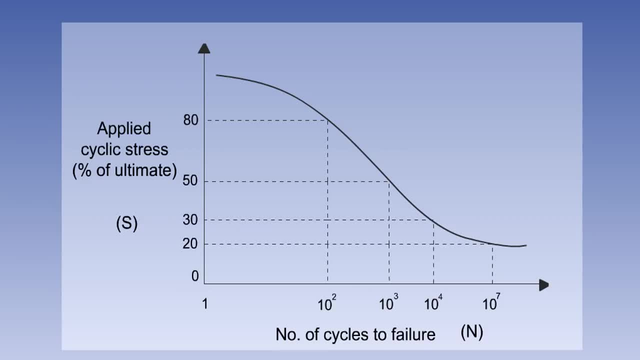 This is a graph of the magnitude of the cycle stress S against a logarithmic scale of cycles to failure N. It can be seen that after 100 cycles, at 80% of the ultimate stress the specimen will fail. But if the stress is reduced to 30% of the ultimate, 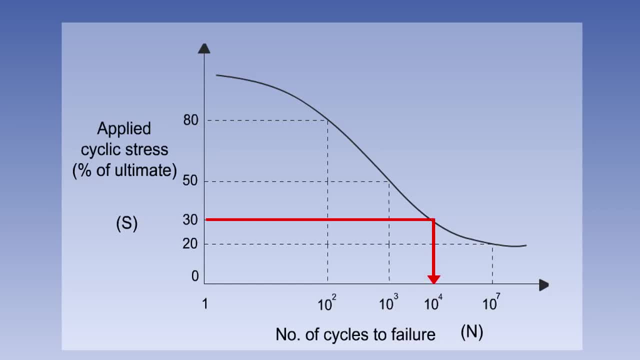 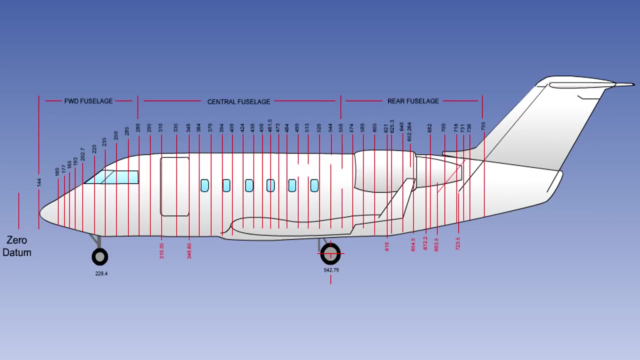 then the component will fail after 10,000 cycles. A method of locating components on the aircraft must be established in order that maintenance and repairs can be carried out. This is achieved by using reference lines to identify positions: fore and aft, left and right and from top to bottom. 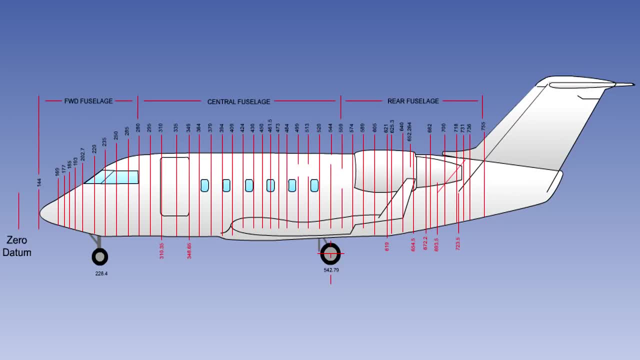 Fuselage station numbers are determined by the number of reversals and determined by reference to a zero-datum line which is at or near the nose of the aircraft. On some aircraft, such as the one shown here, it is forward of the nose. 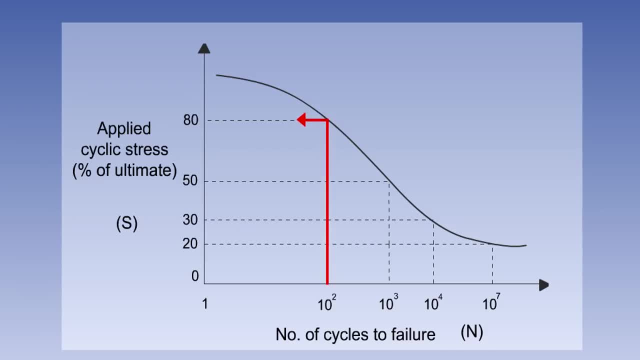 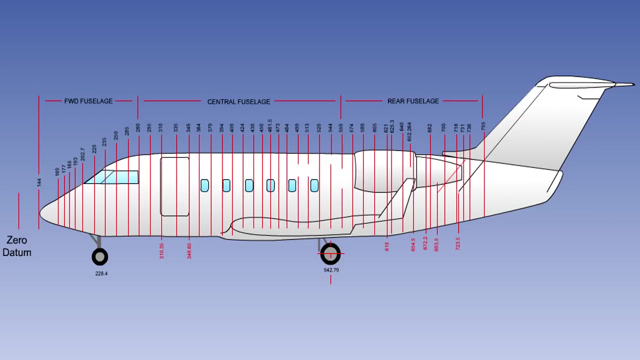 It can be seen that after 100 cycles, at 80% of the ultimate stress, the specimen will fail, But if the stress is reduced to 30% of the ultimate, then the component will fail after 10,000 cycles. A method of locating components on the aircraft must be established in order that maintenance and repairs can be carried out. 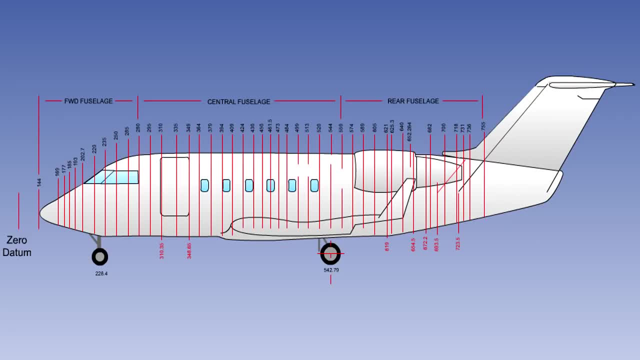 This is achieved by using reference lines to identify positions: fore and aft, left and right and from top to bottom. Fuselage station numbers are determined by reference to a zero datum line which is at or near the nose of the aircraft. On some aircraft, such as the one shown here, it is forward of the nose. 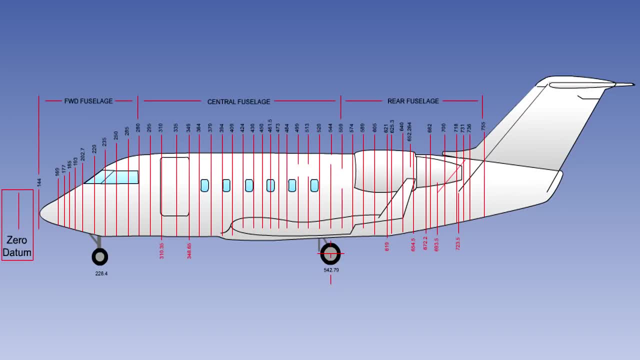 Station numbers are identified in inches or millimetres forward or aft of the zero datum. Stations forward of the datum are identified with a minus sign and aft with a plus sign or no sign at all. In this installation they are all aft of the datum, so no sign is used. 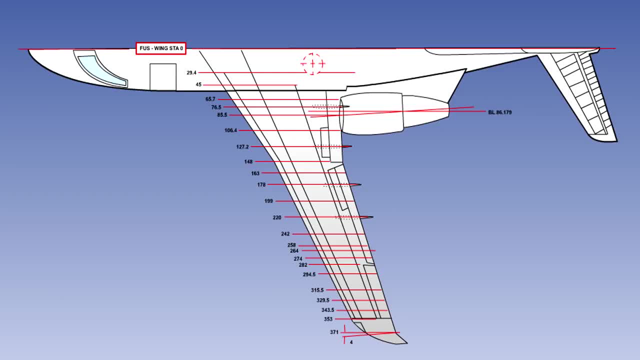 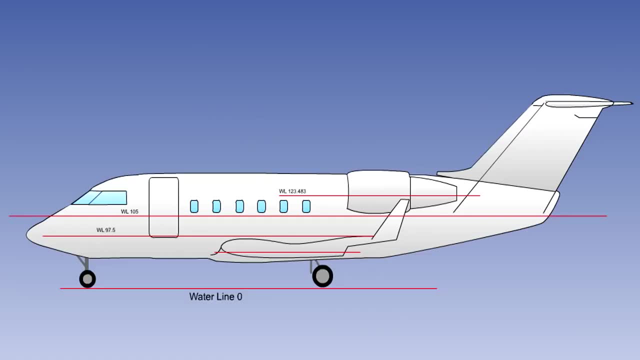 Wing station numbers are measured in inches left or right of the aircraft centre line. Vertical position is identified from the horizontal datum. These positions are known as water lines or buttock lines and are measured in inches from the datum. Plus is used for locations above and minus for locations below the datum. 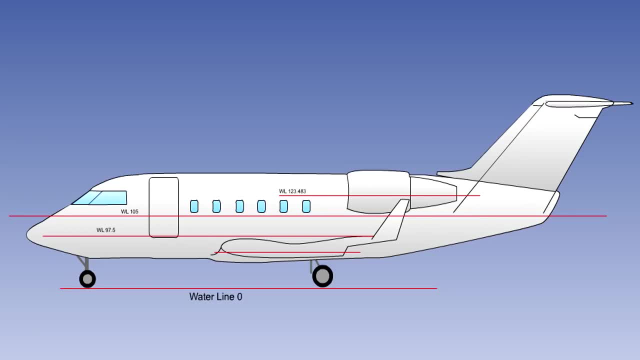 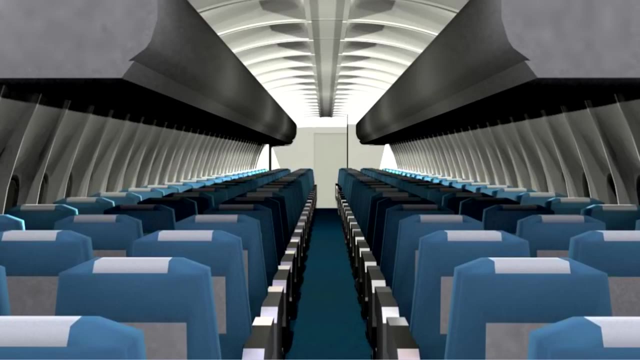 In this example, the datum is at the bottom of the extended landing gear. The fuselage is the main structure of the aircraft. It carries the aircraft payload, be it passengers or freight, as well as the crew, in safe, comfortable conditions. It also provides the crew with an effective position for ejection. 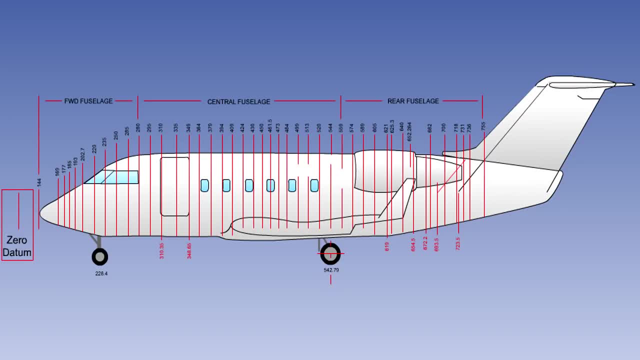 Station numbers are identified in inches or millimetres. forward or aft of the zero-datum. Stations: forward of the datum are identified with a minus sign and aft with a plus sign or no sign, or a minus sign or no sign at all. 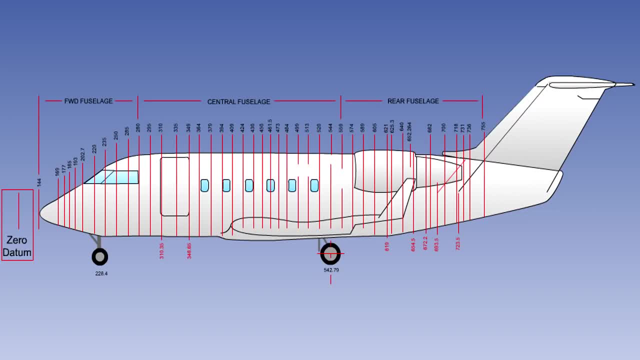 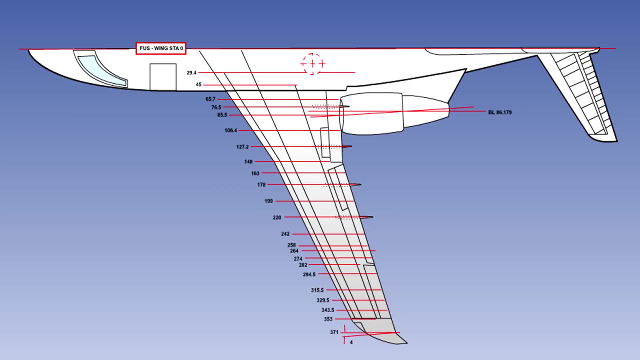 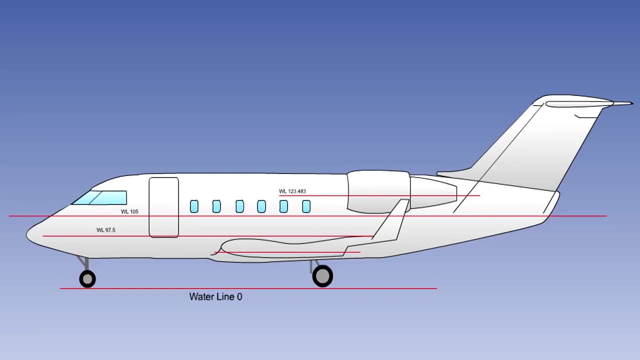 In this installation. they are all after the datum, so no sign is used. Wing station numbers are measured in inches. left or right of the aircraft centerline Vertical position is identified from the horizontal datum. These positions are known as water lines or buttock lines and are measured in inches. 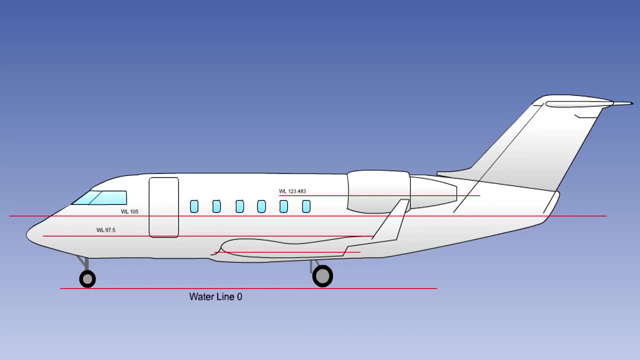 from the datum. These positions are known as waterlines or buttock lines and are measured in inches from the datum. Plus is used for locations above and minus for locations below the datum. In this example, the datum is at the bottom of the extended landing gear. 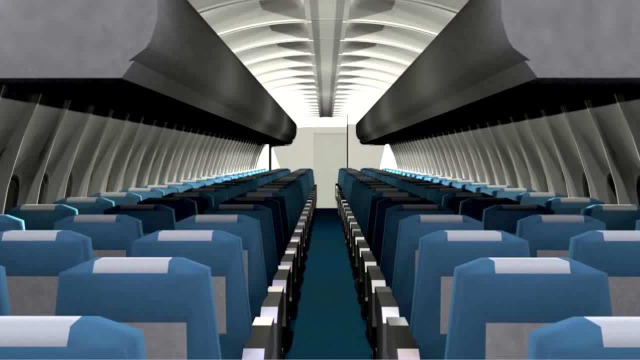 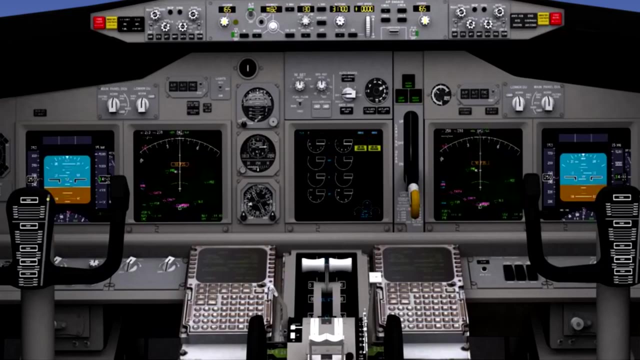 The fuselage is the main structure of the aircraft. It carries the aircraft, payload, be it passengers or freight, as well as the crew, in safe, comfortable conditions. It also provides the crew with an effective position for operating the aircraft and space for controls, accessories and other equipment. 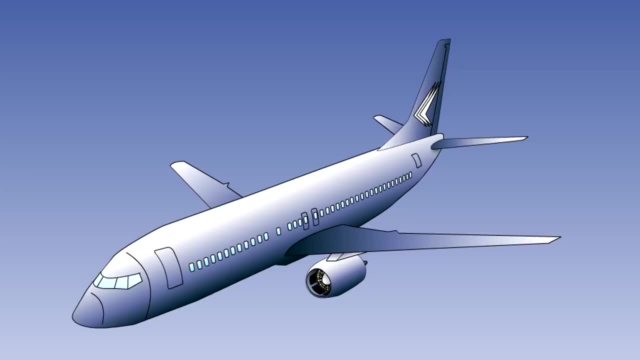 The fuselage transfers loads to and from the wings, tailplane, fin landing gear and in space, In some configurations, the engines. Modern aircraft fuselages are pressurised and these pressurised aircraft structures must also be capable of withstanding axial and hoop stresses imposed by the pressurisation. 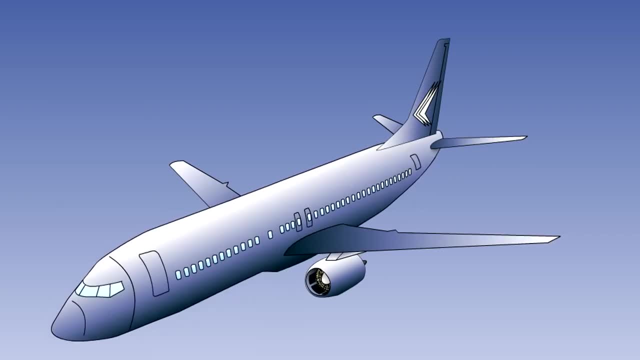 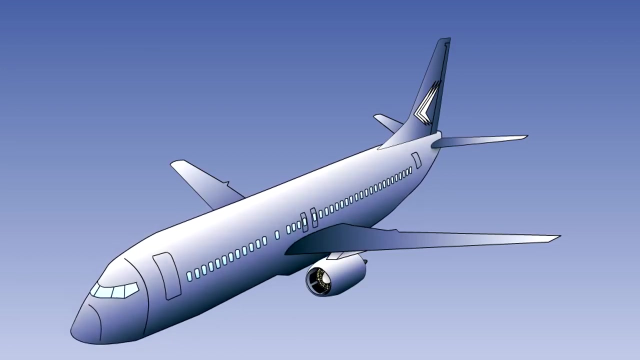 forces. Axial or longitudinal stresses are set up in the fuselage of aircraft when pressurised and tend to elongate the fuselage between the front and back, The beggedальный and rear pressure bulkheads. Hoop or radial stresses, also caused by pressurising the fuselage, tend to expand the fuselage cross-section.